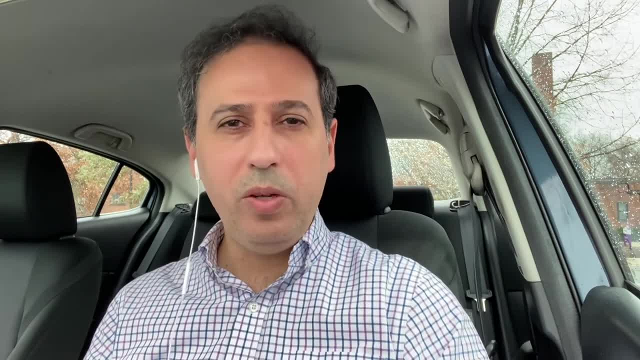 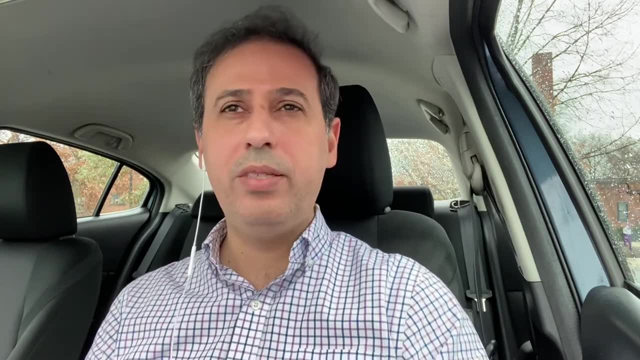 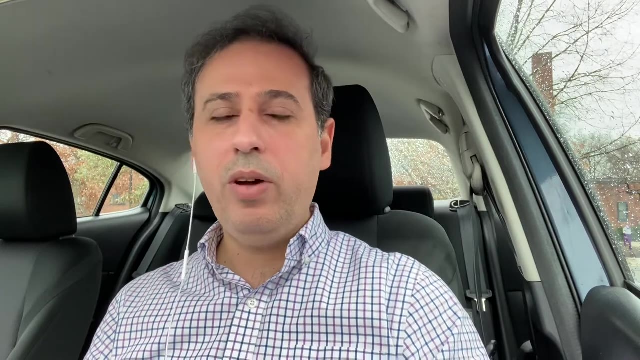 the notification bell so that you get informed every time. you know once when I upload my videos and before I answer the question, which is very important, that I hope that you will stay till the end of the video to know the answer and you watch the whole video and within it, with its entirety. so I would like to give a 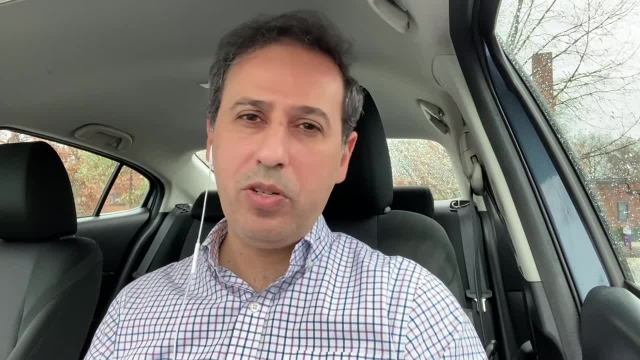 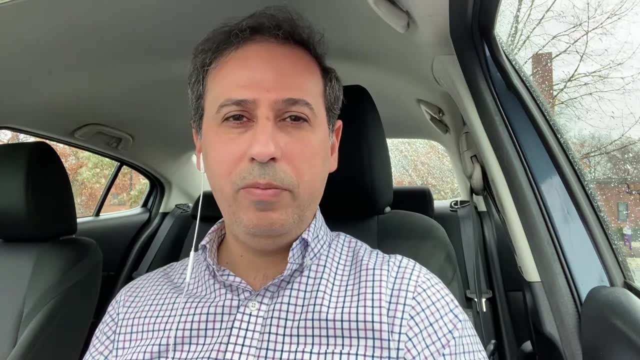 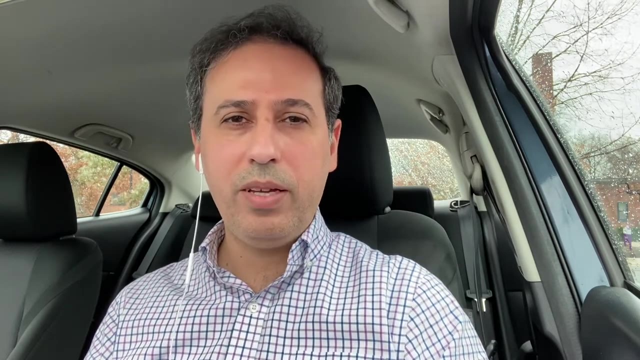 shout out to one of my websites that I am actually managing and the proud owner of which is for Petracom. Petra is a World Heritage Site in Jordan, in the Middle East, and it is also one of the new world wonders. I will leave a link for my website in the description. 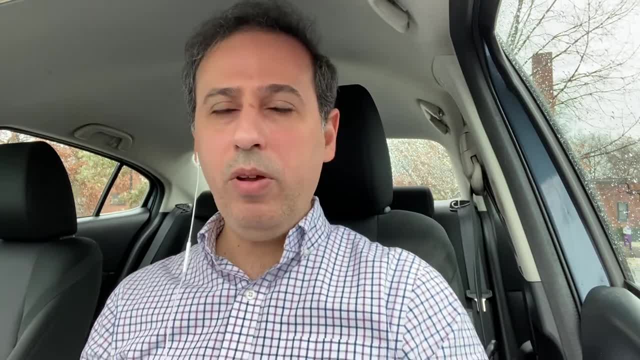 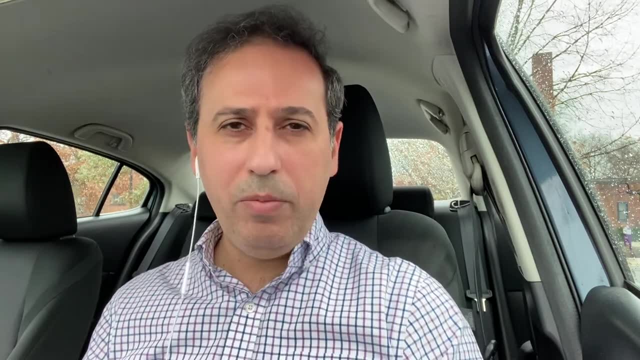 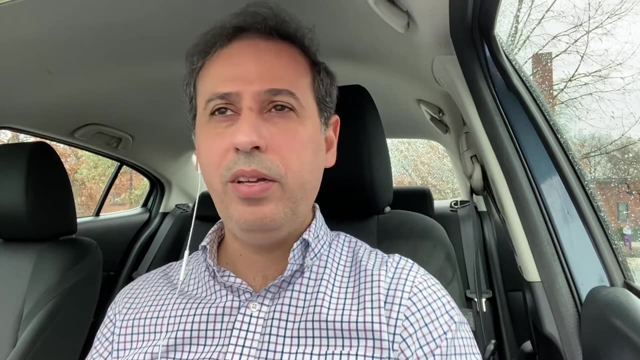 go and check it. it's worth checking there. now we're going back to the question. so I receive a lot of questions from my- you know- students and my friends and family members who their kids or you know children, are interested in studying biomedical engineering, asking what is the best field to study and to focus on in biomedical engineering. so and 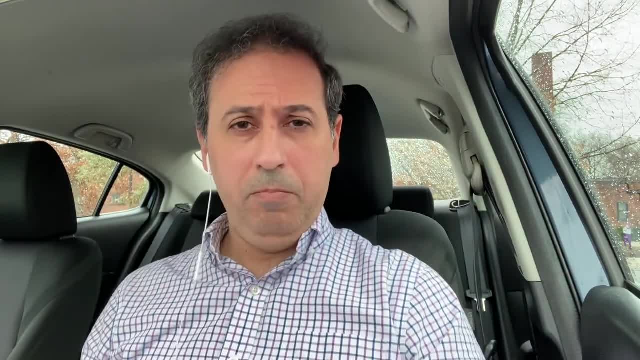 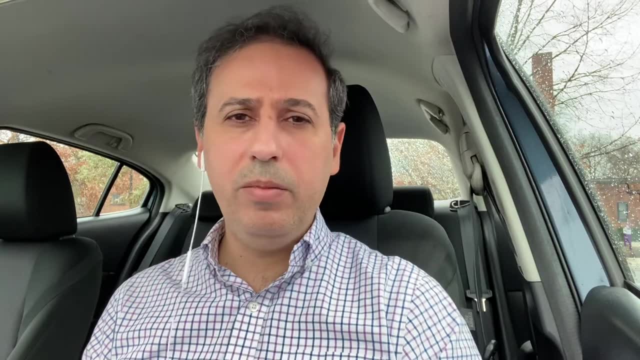 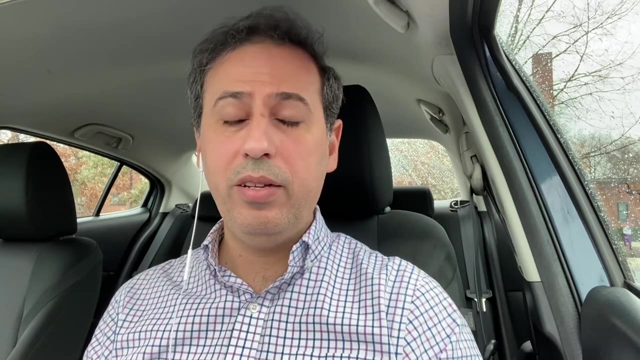 especially, you know, engineers who are, you know, newly graduated and they would like to invest their time in a graduate school and they would like to find out what is the field that they the best you know in biomedical engineering, for them to invest their time, money and energy, and that is, and also which is, rewarding. 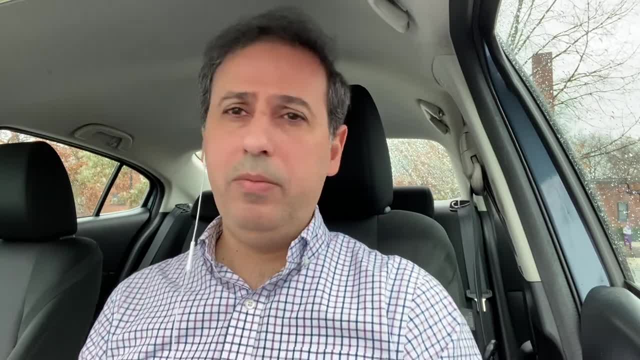 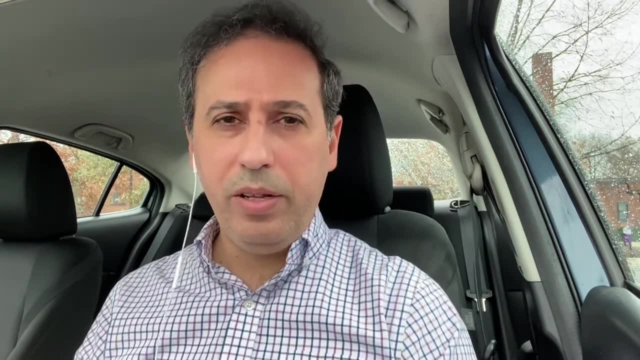 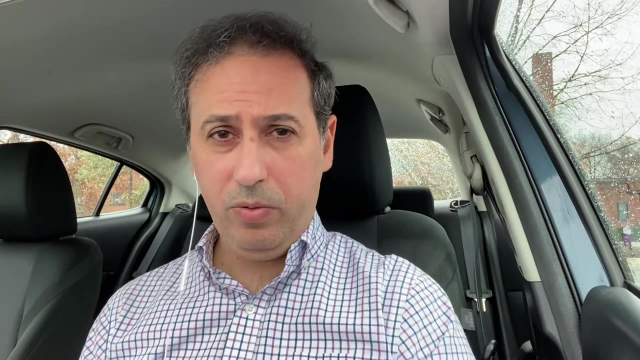 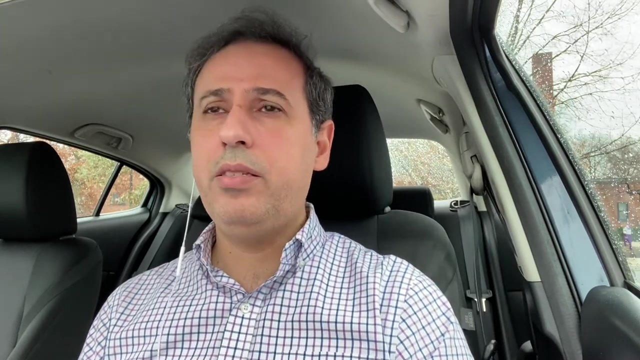 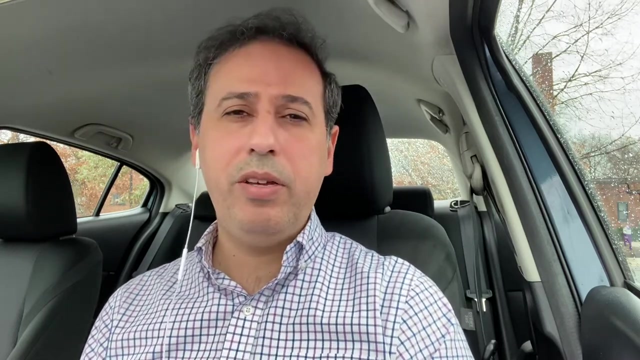 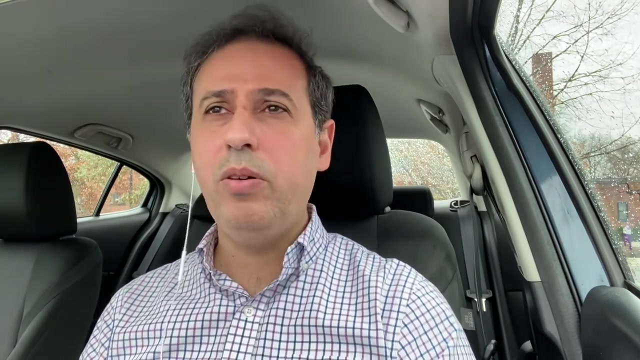 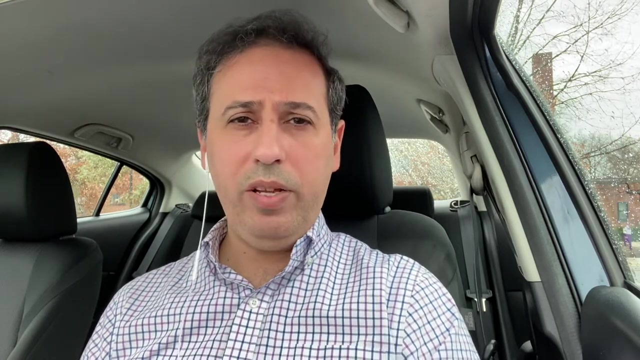 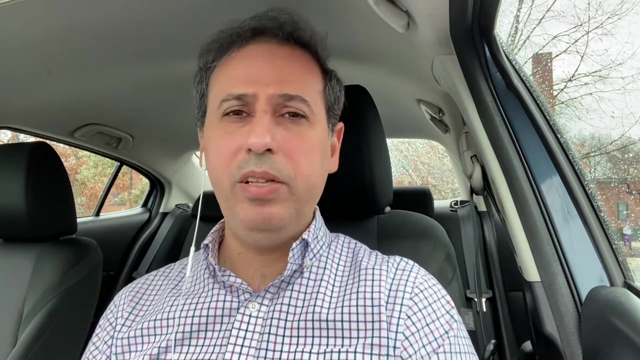 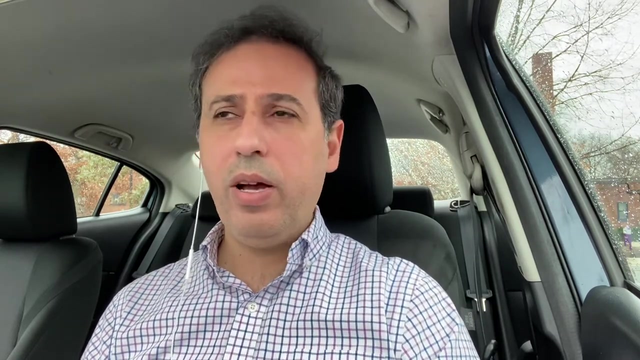 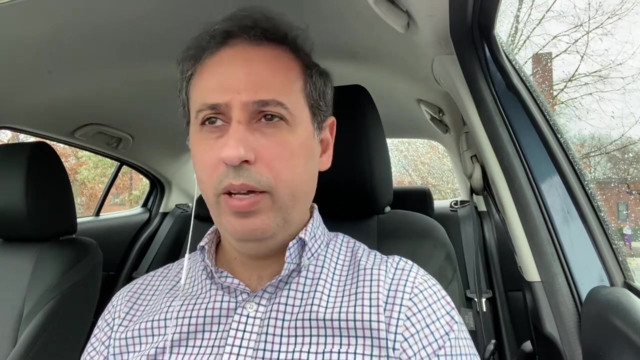 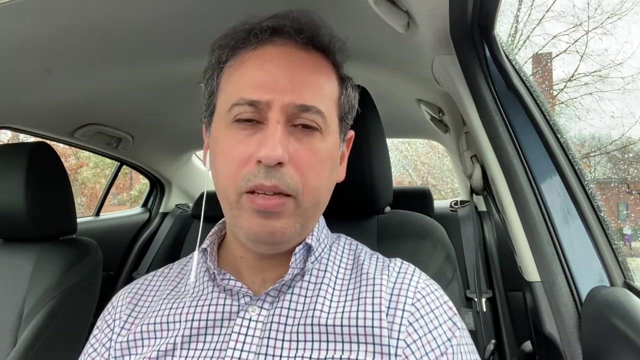 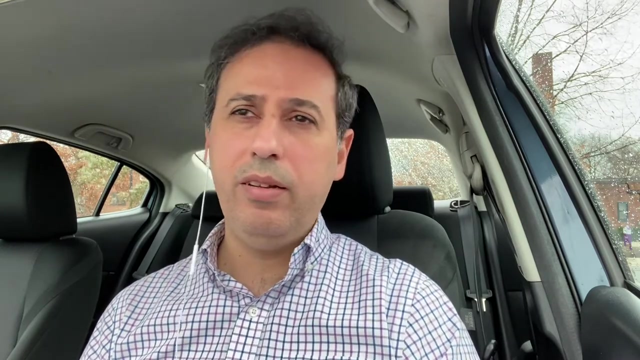 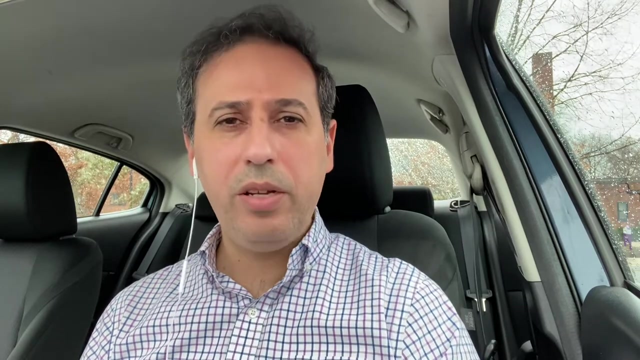 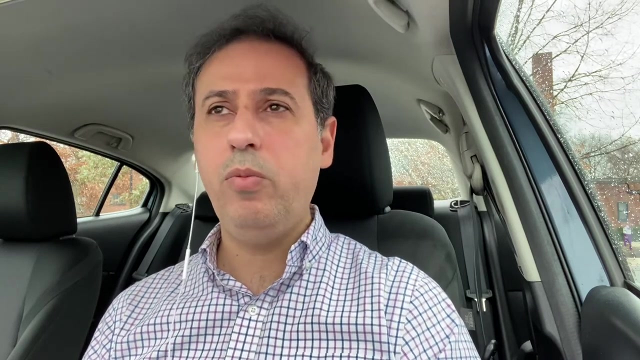 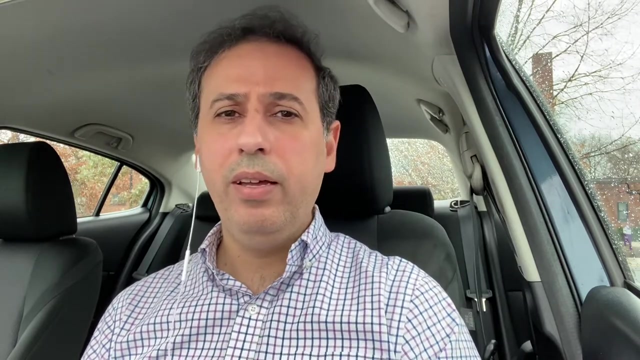 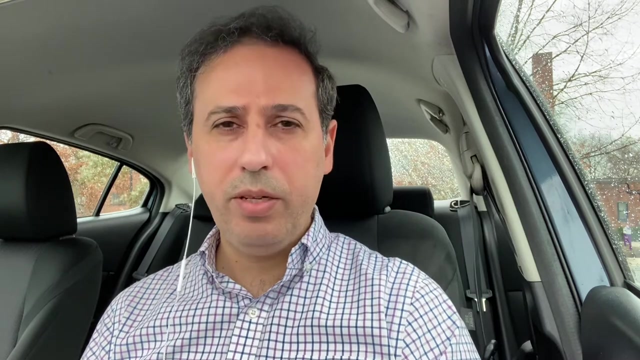 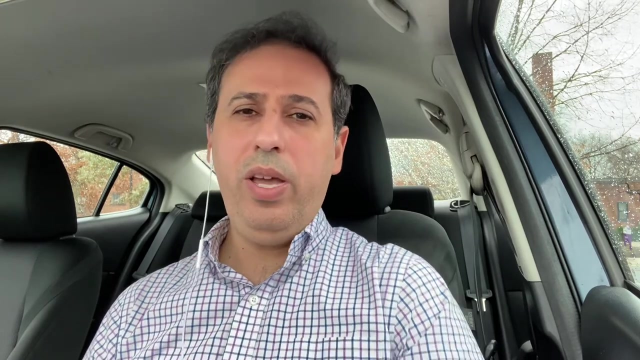 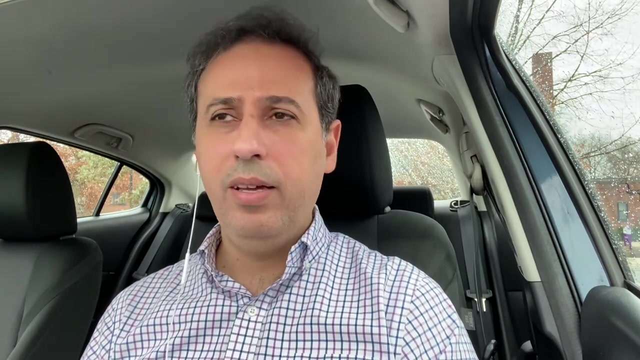 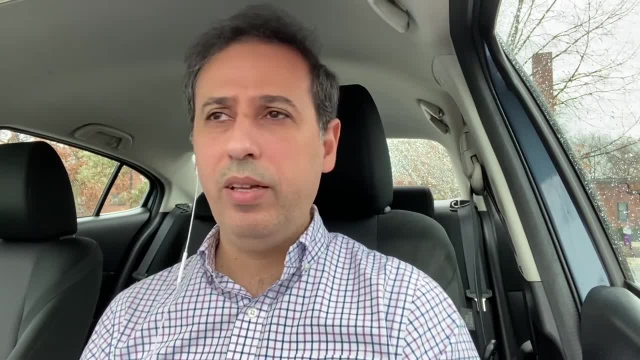 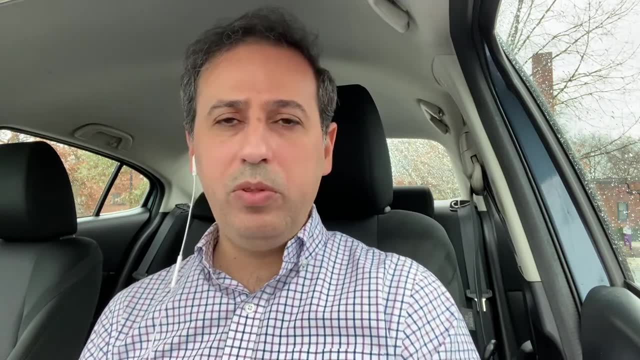 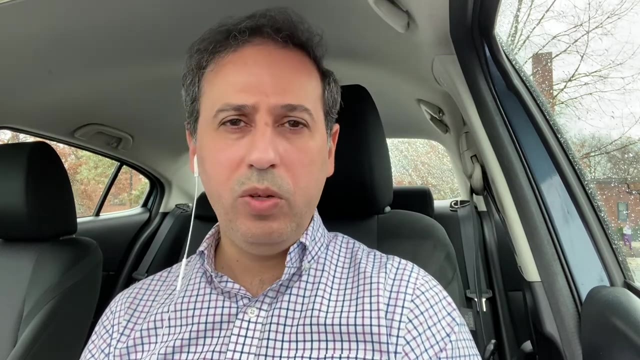 best and also we have. we can add to it 3d printing, even biological 3d printing. So the field is expanding and growing and we come down to this question: which one of them is the best to invest your time, money and energy and to make it as a you? 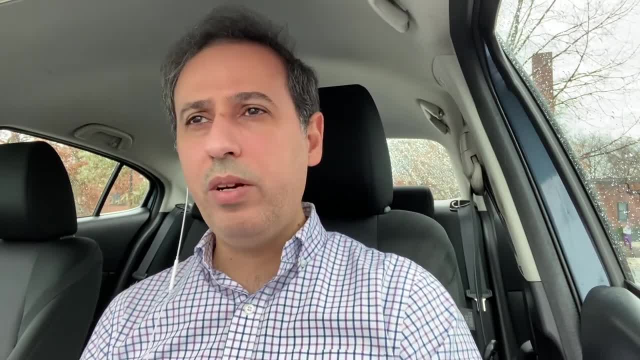 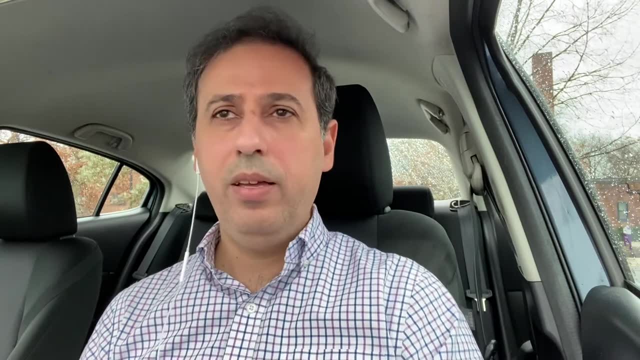 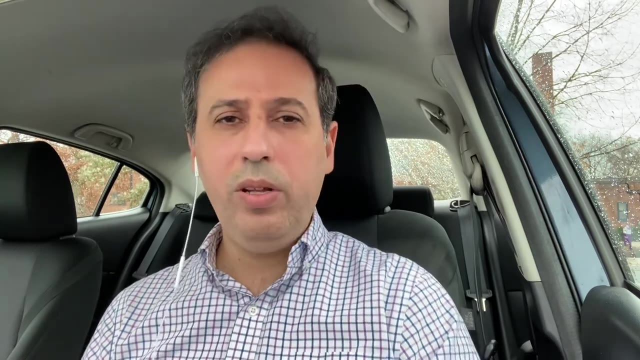 know the core of your profession, And that is where my answer to my students and everybody who ask this question is: go back to your, to one question. Asking which field is better is not the right question. We need to ask another question that will help us. help us. 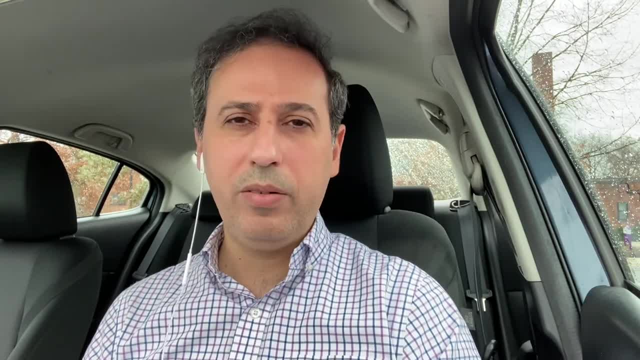 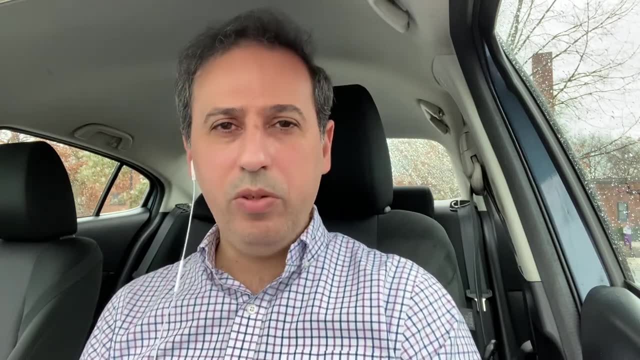 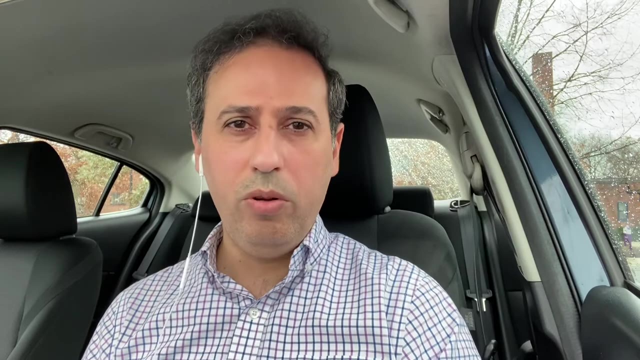 a lot in in deciding which field is better and why. The question that I'm proposing to everybody to think of is this: what is the medical condition or the medical challenge or the medical problem that you feel passionate about and you would like to solve and to help solving, and that has some kind of 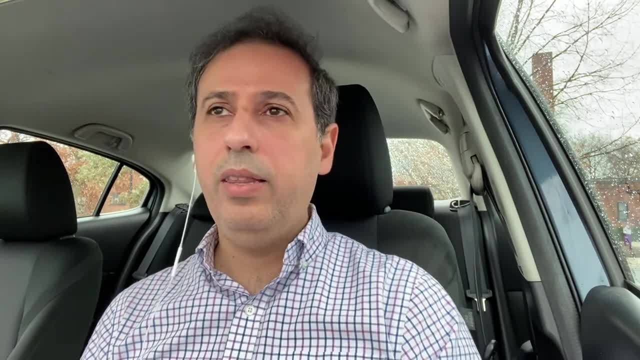 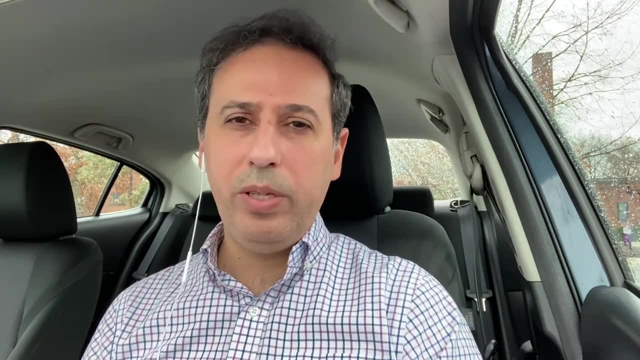 personal. you know experience with you. This is the right question. Once you answer that question, you know exactly which field you want to be in. So, instead of asking which field in biomedical engineering is better for you know, graduate school or for better for me or for is better for making money? the 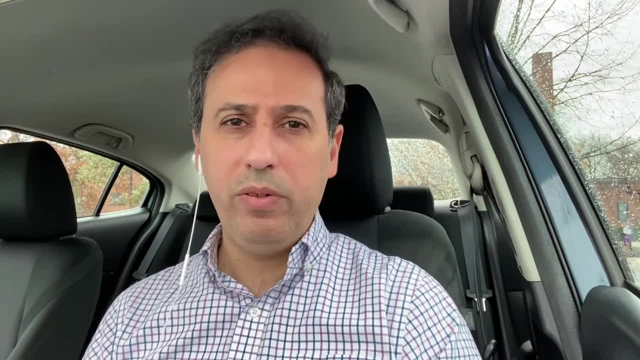 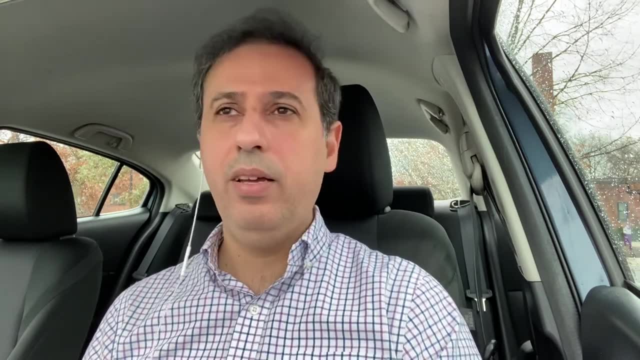 question is: what is the medical condition that you would like to solve or medical challenge that you would like to participate in solving? That is the best. that's a much better question to ask and to me- I am a- you know, I'm a bone guy. I. 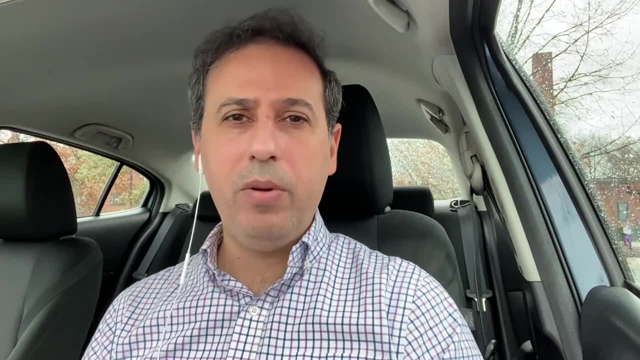 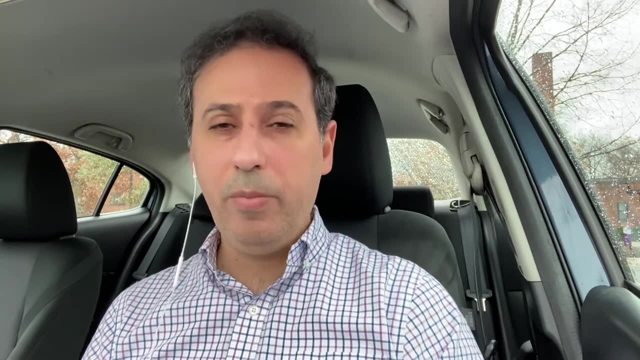 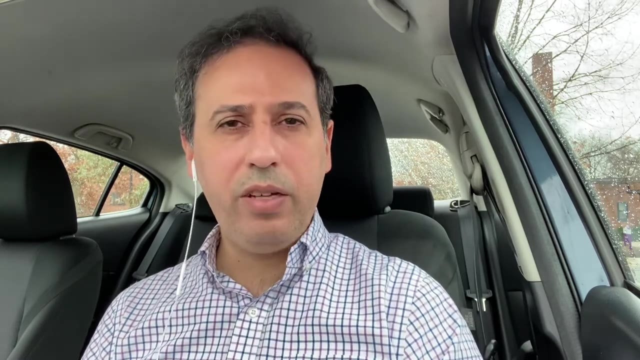 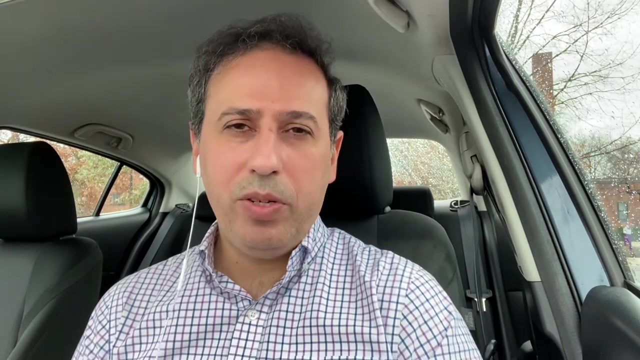 worked all my life in bone. I feel passionate about creating solutions for people who suffer from fractures and they're diabetic as well as osteoporotic. So I focus on osteoporosis and diabetes and its effect and that you know they're deteriorating effects on bone and that is my. that's my passion. 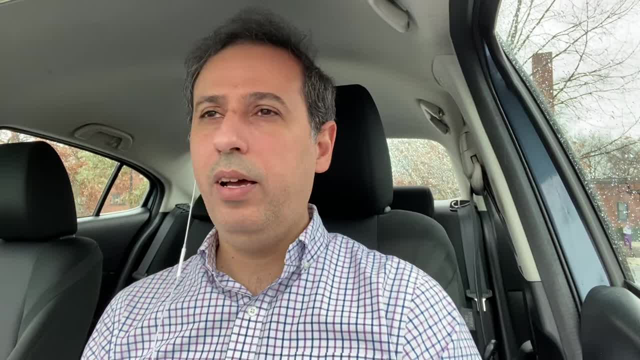 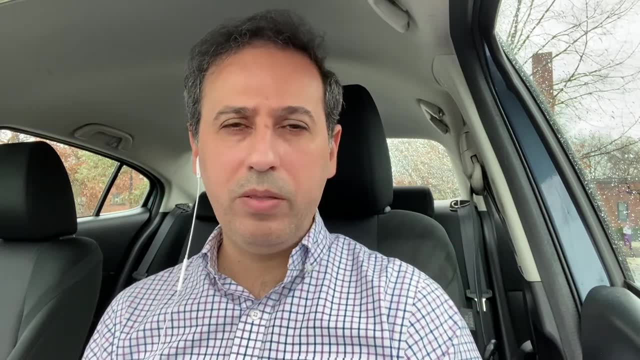 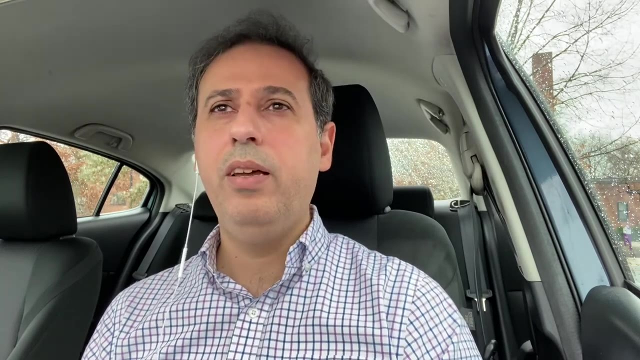 because I know that we have a lot an aging community society. people live longer and they want to be active and productive and they want to be independent, as you know, long as possible. Diabetes actually affects not only our metabolism, but it also affects the anabolic action. you know activities and anabolic processes of bone, as well as 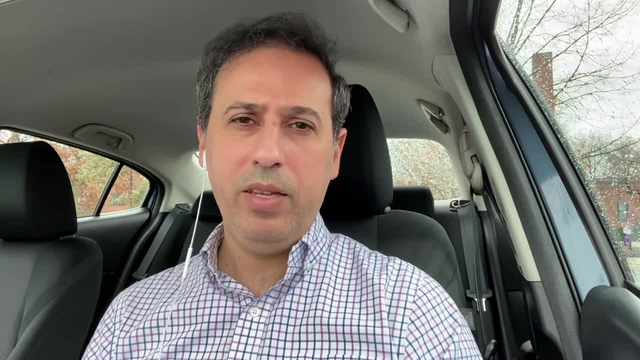 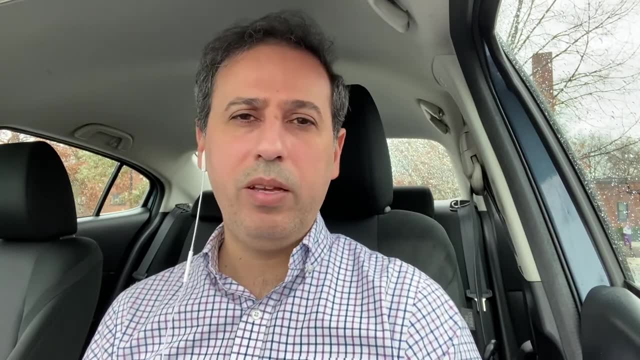 skin. So if you have someone is diabetic and they experience a cut in the skin, it will take twice the time to heal- if it healed and also if it's going to heal. and also the same thing goes for bone. So a diabetic person will with a fracture. 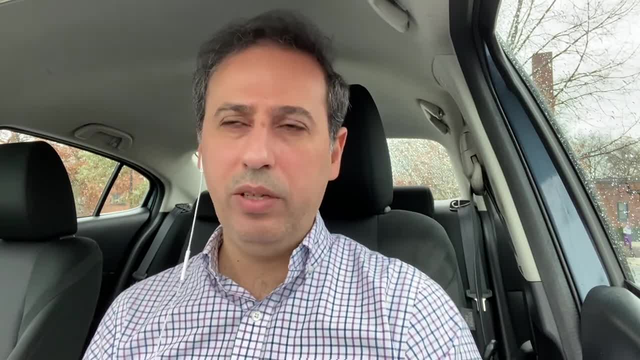 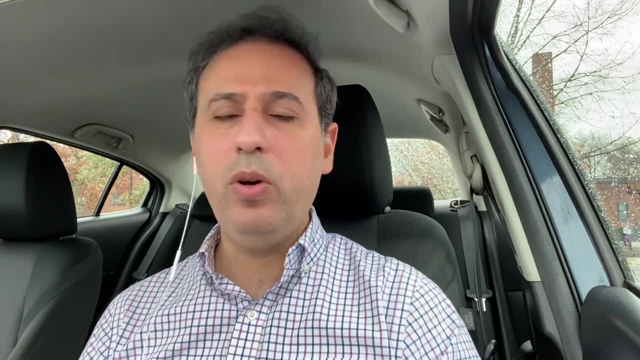 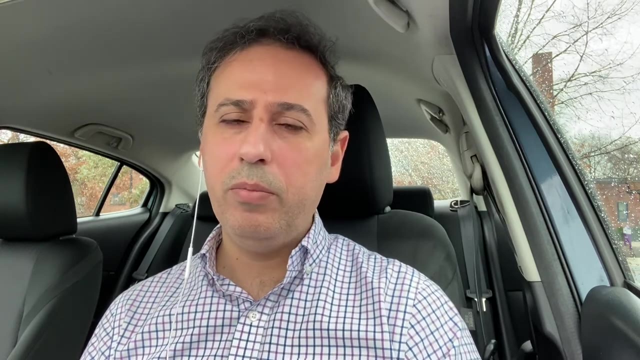 the bone will not heal as it's supposed to heal- In the same way that it's a normal person would- actually The bone of a normal person would- And also osteoporosis is a huge problem within our aging communities. So what I wanted to invest my time and energy in is 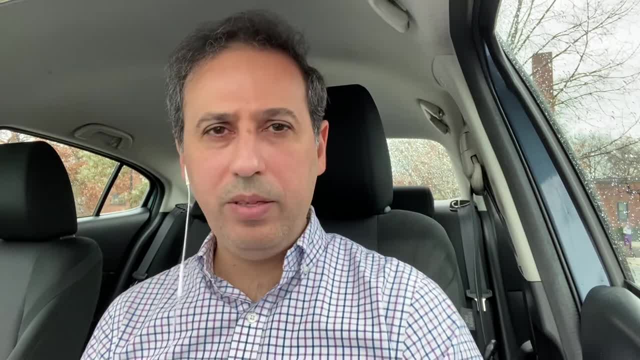 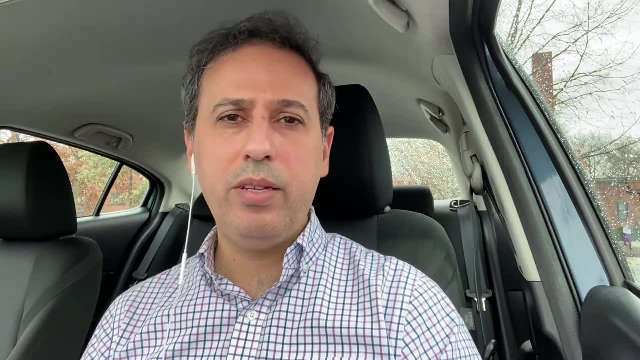 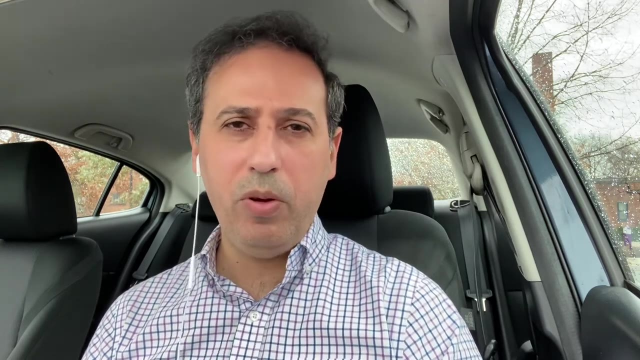 learning everything I can in order to help solve this, these two, the challenge of bone regeneration and bone healing in the presence of osteoporosis and diabetes- And, by the way you know, diabetes is a prod dependent in females because of the menopause. 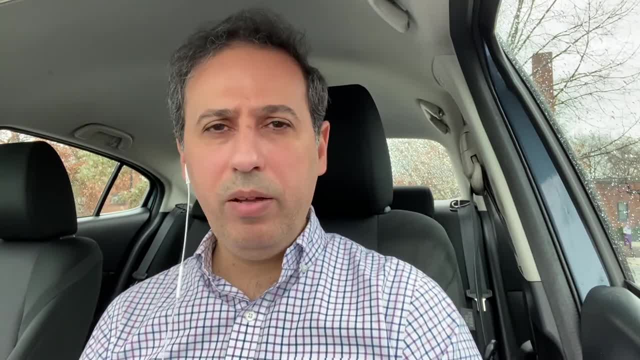 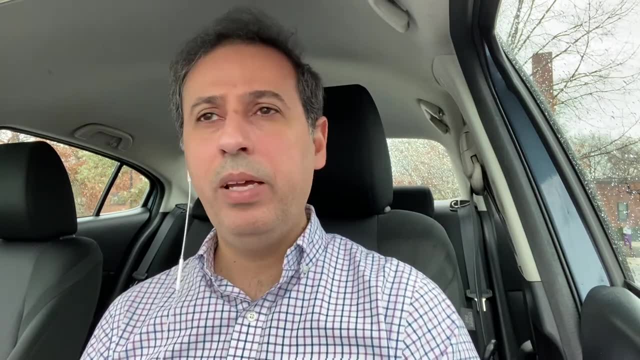 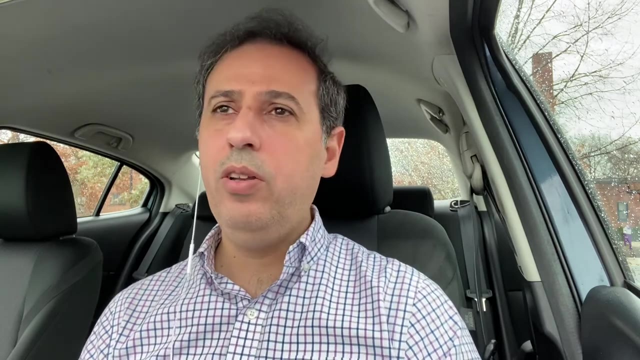 their hormonal cycles. For men, for males, diabetes actually can result in osteoporosis. So it's it's a complex problem and I would like to, I want I learned everything that I can in order to help people. So how did I approach this? I know how to use mechanical testing to this bone. I, as an engineer, I. 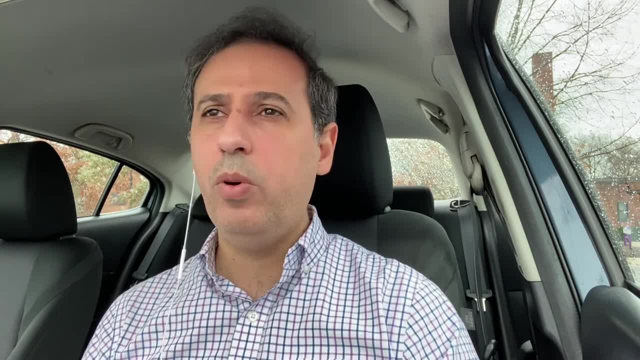 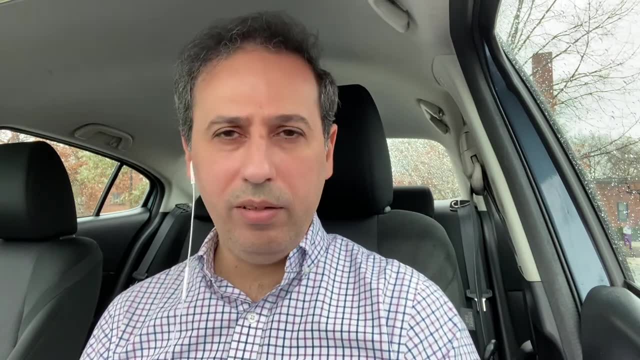 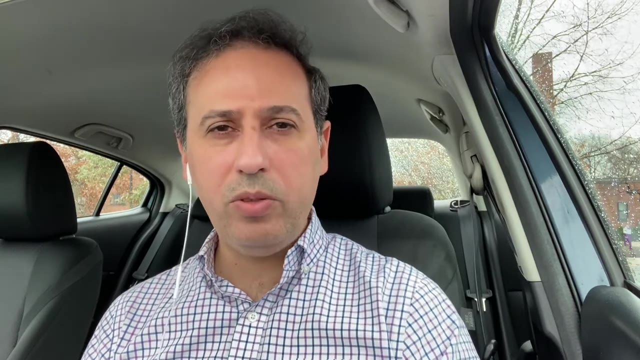 know how how bone actually forms aisi and how bone metabolize, and also how bone regenerate in the case of you know fracture. i know all the cell cells involved in the bone tissue. i know how they work, how they function. i know how to use ultrasound to accelerate bone healing. i know how to use electromagnetic waves. 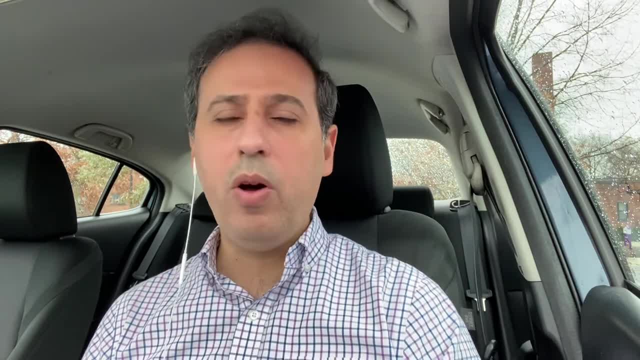 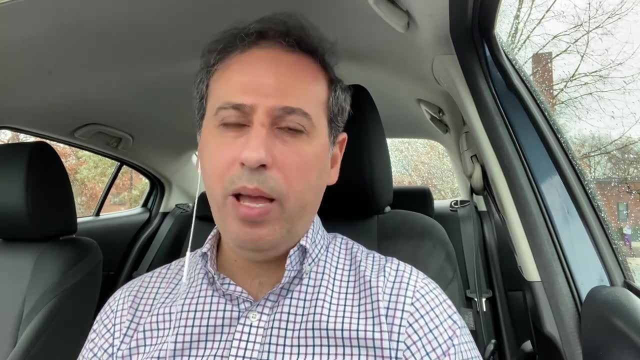 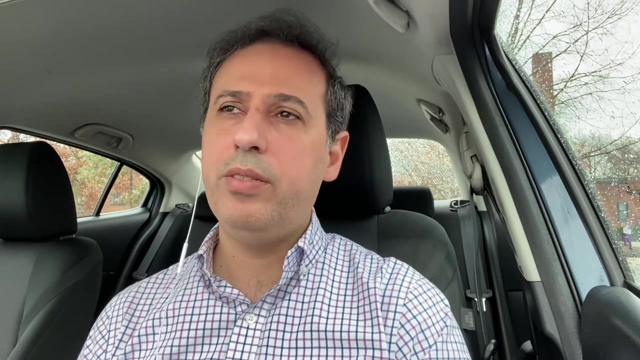 to accelerate bone healing. i know how to design robotics and how to program arduinos for assistive technologies. you know rehabilitation engineering, so i'm i mean as an engineer. my challenge is clear, which is the effect of diabetes and osteoporosis on bone and bone metabolism, and 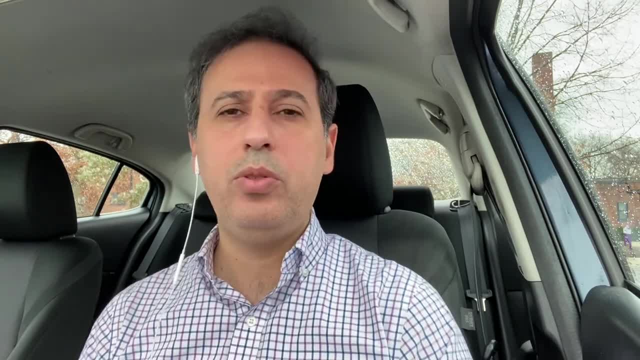 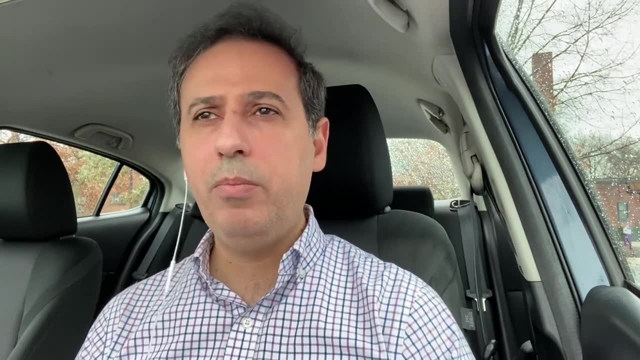 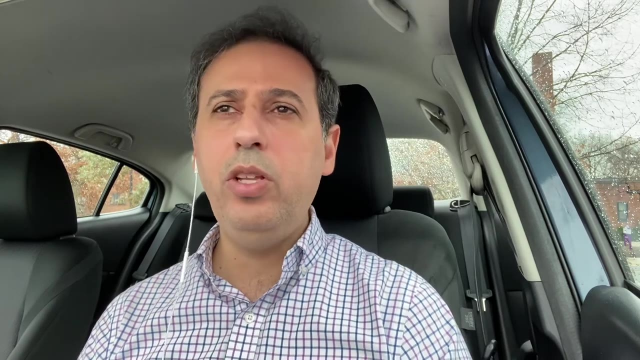 bone regeneration, and i invested my time in order to try to solve this medical challenge, and that's what i want you to think of. i want you to think about what is the medical problem or medical challenge that you feel passionate about and it touched you personally and you would like to solve, and then you need to learn everything. 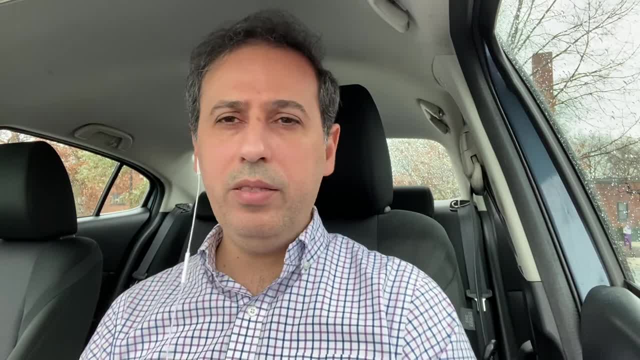 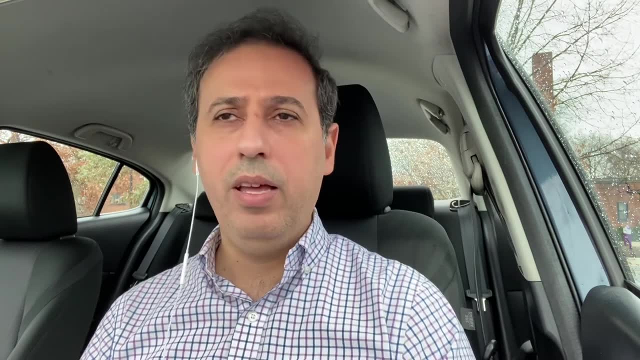 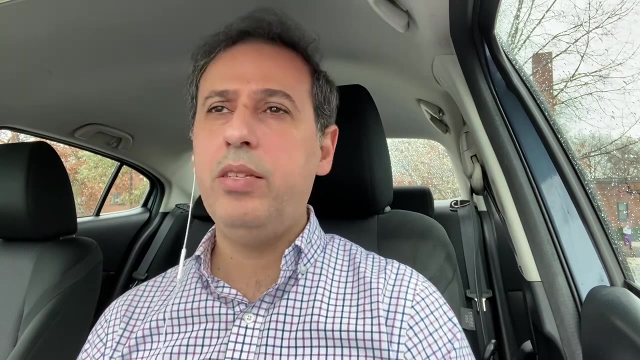 in order to solve that medical problem. this is a much better approach actually for biomedical engineers to identify which field they want to be in and as you progress in your learning and in your training, as well as a new profession you will be, you know exactly what is. 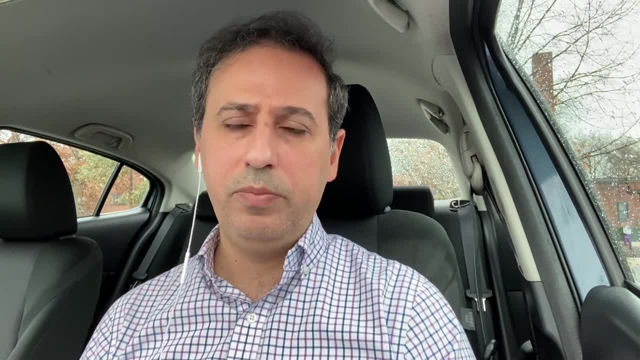 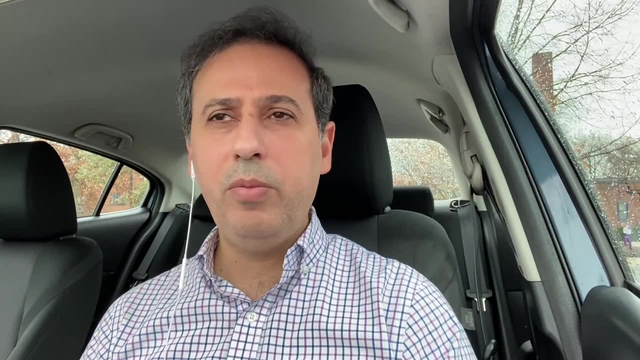 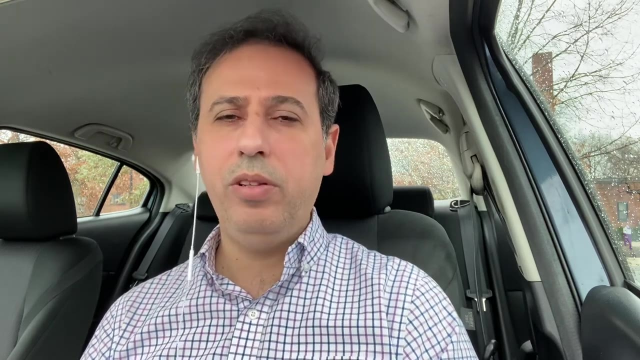 the thing that you want to do and which field is better for you. so i hope that's helped and in identify, in helping biomedical engineers or biomedical engineering students or whoever is interested in biomedical engineering to you know, focus on what they actually feel passionate about by identifying what is the medical problem. and one thing before we i leave: